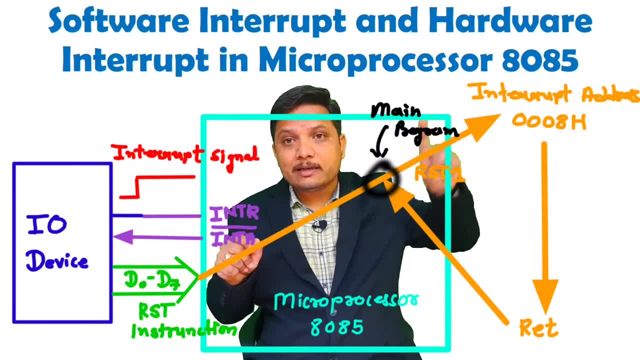 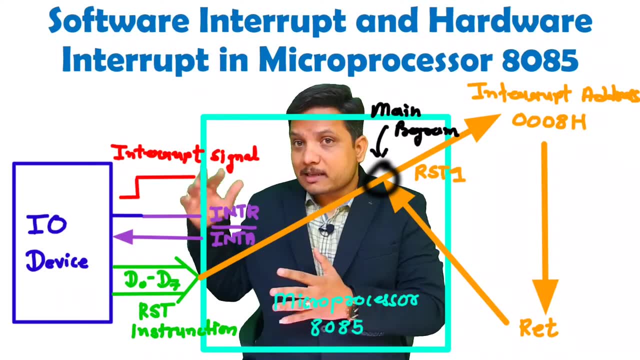 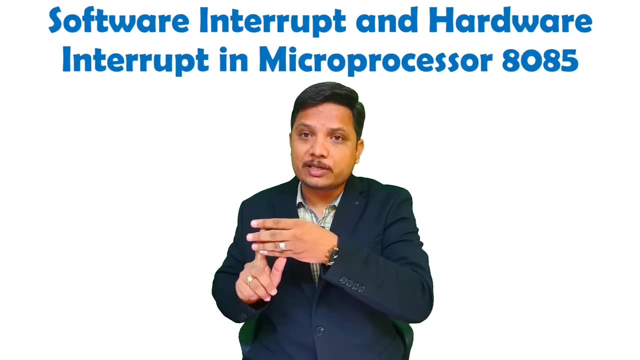 microprocessor will transfer it controls to that service routine. So interrupt, interrupt Interrupts are given by external devices only. but in hardware interrupt all the pins are having well-defined memory location for that service of interrupt. But when it comes to software interrupt, at that time interrupt will come from hardware. 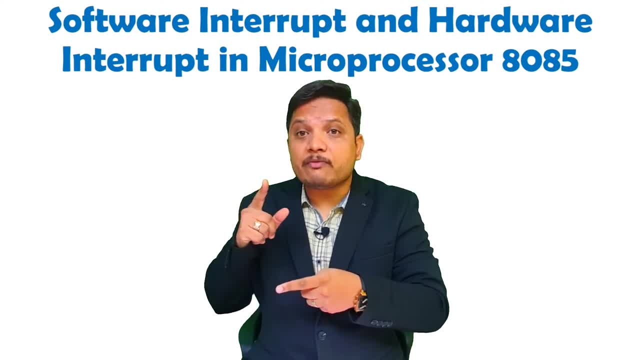 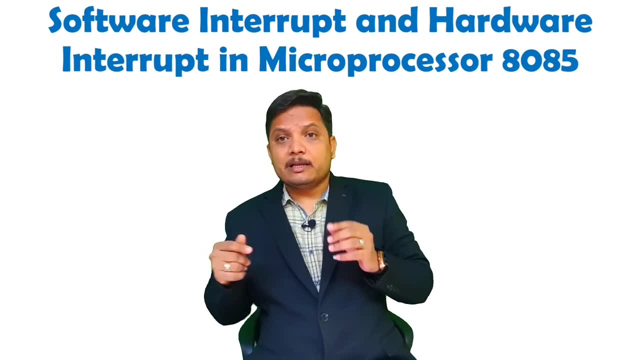 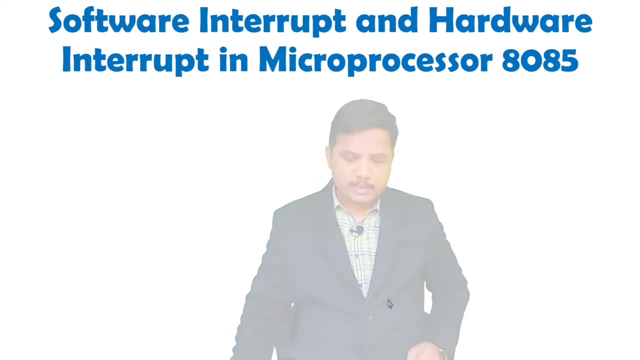 But here instruction of transfer of control, that will be also given by that hardware. So that is how it is different. right Now, my dear students, let us try to understand all those things step by step, so that we will get more clear in terms of comparison. 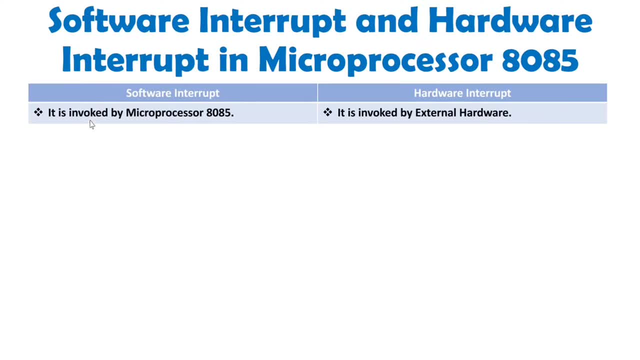 So when we talk about software, interrupt, so that is invoked by microprocessor 8085.. How it is invoked by microprocessor 8085?? Once microprocessor 8085 receives instruction and when it executes that instruction, at that time interrupt service will get provided. 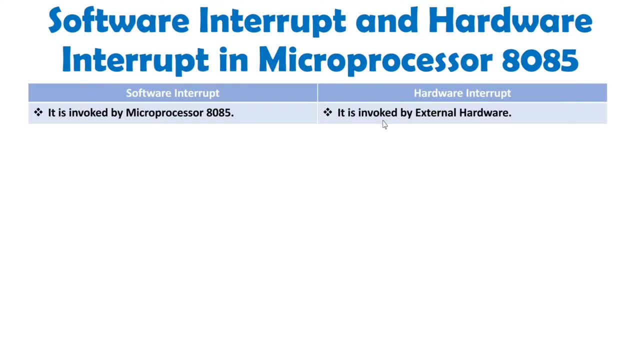 And here Hardware interrupt that is invoked by external hardware. How, Whenever external hardware is providing interrupt, at that time pin will directly transfer control to the interrupt service, As all the hardware pin are having well-defined memory location. I will explain you even how. 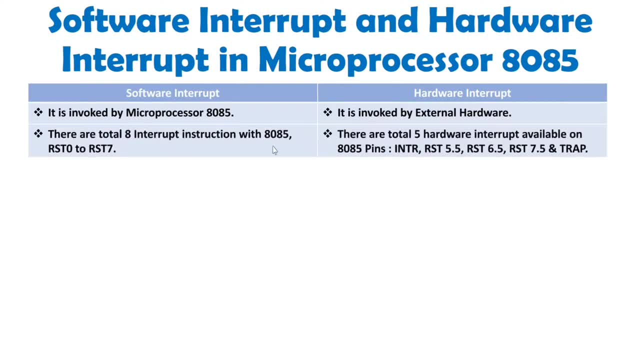 those memory locations are there. When it comes to software interrupt, then microprocessor 8085 is having total eight interrupt instructions. Those instructions are RST 0 to RST 7, and with hardware interrupt there are a total five pins available with 8085,: INTR, RST 5.5,, RST 6.5,, RST 7.5, and TREP. 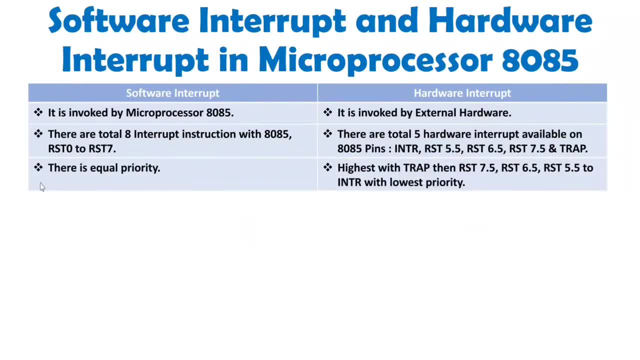 When it comes to priority, then in software interrupt all interrupts are having equal priority. Why? The reason is: 8085 can execute only one instruction at a same time. So that is why it is called RST 0 to RST 7, and with hardware interrupt there are total. 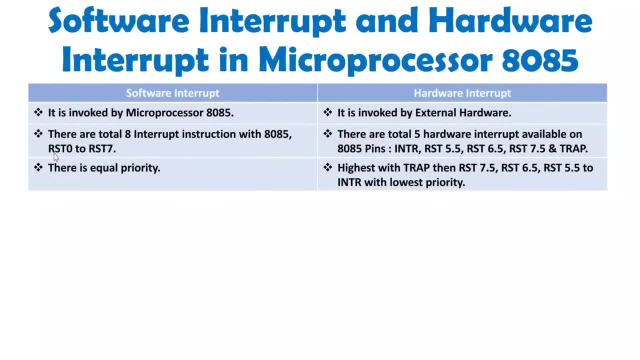 eight interrupts available with 8085, INTR. RST 5.5, RST 6.5, RST 7.5,, RST 6.5, RST 7.5, and TREP, So RST 0 or RST 1 or RST 2 or RST 7 can be executed. 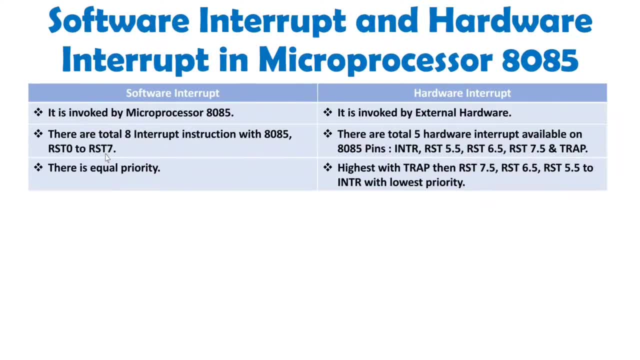 It cannot have execution at the same time. right, So all are having equal priority. but in hardware interrupt it is possible that multiple interrupt may occur at the same time. Then highest priority, that is given to TREP. After that priority is there with RST 7.5, then RST 6.5, RST 5.5, and lowest priority. 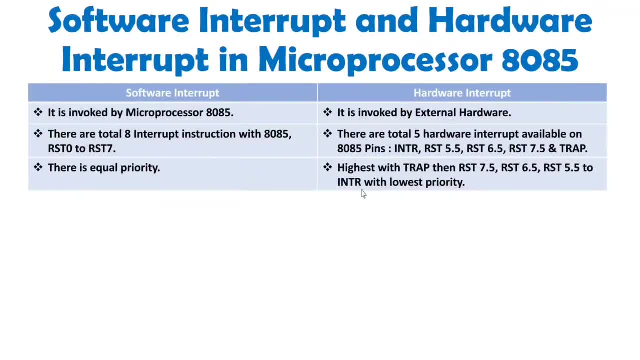 that is assigned to INTR line. So that is how priority is defined, with hardware interrupt and with software interrupt. My dear students, when we talk about triggering, then with software interrupt, interrupt is getting triggered by instruction execution right. But in hardware interrupt you will be observing that triggering will happen with respect to 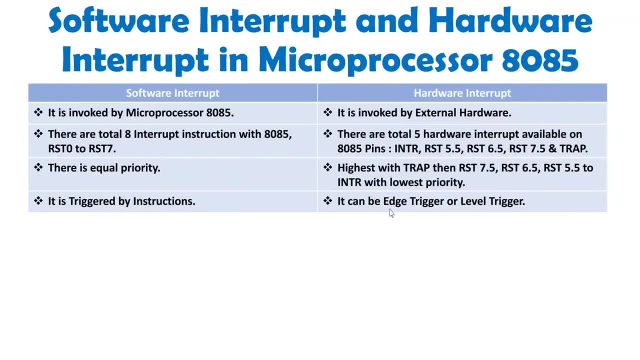 signal and that signal may be edge trigger signal or it may be level trigger signal. You see, edge trigger means whenever signal goes from low to high, So low to high transition. that is referred as edge trigger signal. But when it goes from low to high, but triggering will happen when it stays high. 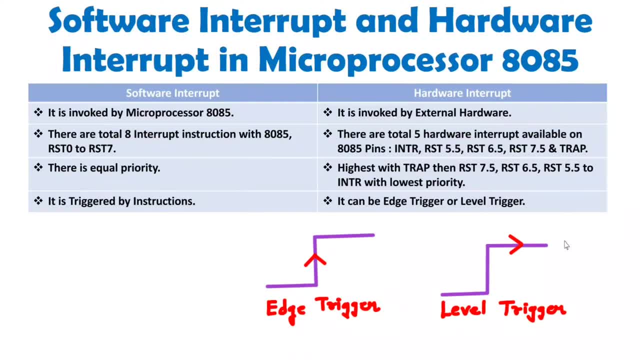 That is referred as level trigger signal. I'll explain you that in detail when I explain you: hardware interrupt Now when we talk about disabling of interrupt. so at that time you should know, my dear students, we can disable all software interrupt by DI instruction, as well, as there are many other. 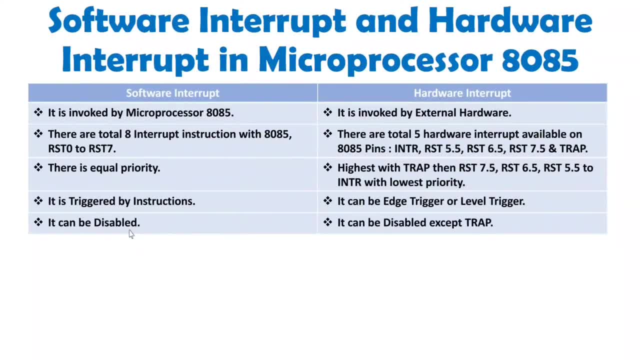 ways by which we can disable interrupt, that we will discuss in Interop of 8085 main block diagram. Now, when we talk about disabling of hardware interrupt, then other than trap can be disabled. Now let us talk about how locations are there with interrupts. 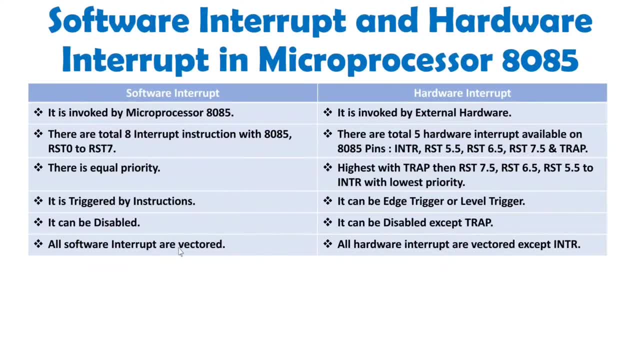 So all instructions which are there with software interrupt, those are vectored. Vectored means all the instructions will transfer control of program to the well defined memory locations. So that's why all software interrupts are vectored interrupts And with hardware interrupt. my dear students, you should know that other than I and TR are 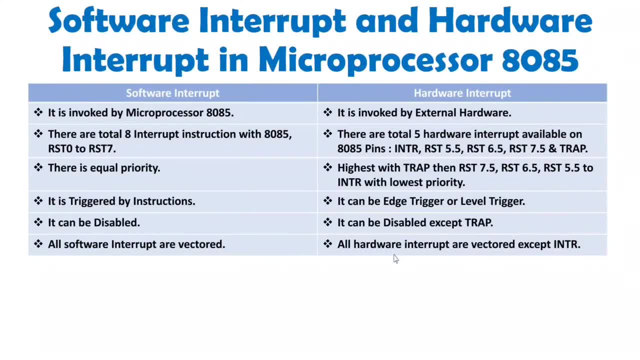 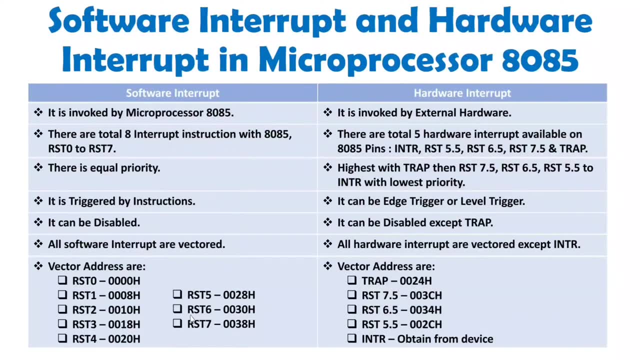 having vectored address, And let us see what are those locations. even So, when we talk about RST zero to RST seven, then you see we have well defined memory location with each instruction execution, as if you execute RST zero, program control will get. 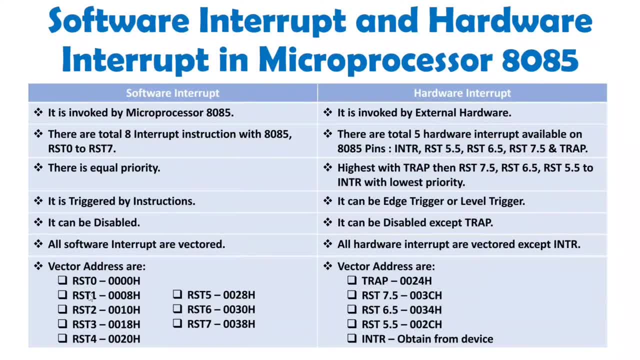 transferred to 0000 hexadecimal. Okay, When you execute RST one program control will get transferred to 0008 hex. Likewise, addresses are there and you can easily remember these addresses. even You see, RST zero is having 0000, then you will have to add eight. 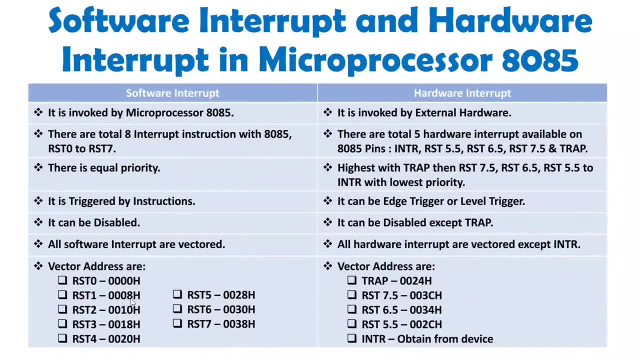 So RST one is having 0008 hex. Then if you add eight, then RST two address will be there, That is 0010 in hex. In hex you will have to do this addition, Remember this. and you can have RST seven with address 0038, as per the addition in sequence. 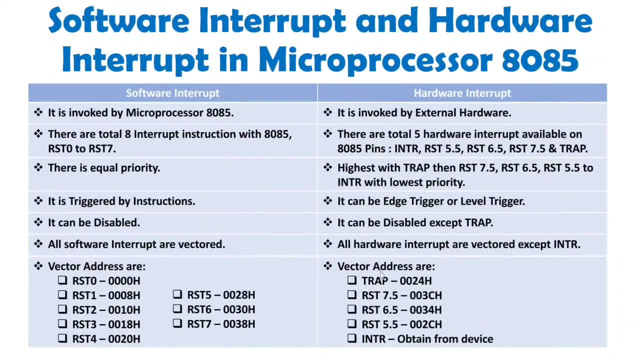 by eight. Now when we talk about vector address of this hardware- interrupt- then this trap is having address that is 0024 hex. Now how to remember this. See, initially trap was named as RST 4.5.. Now how to remember this. 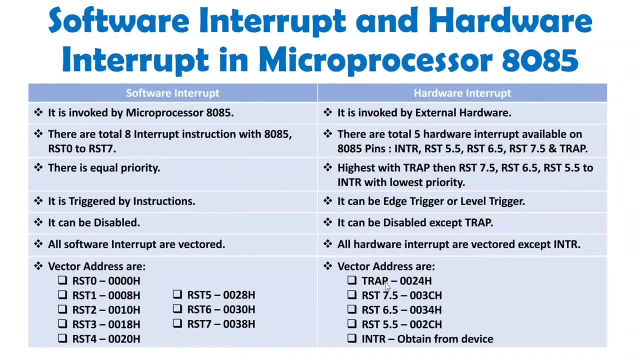 See, initially, trap was named as RST 4.5.. Now, how to remember this? See, initially, trap was named as RST 4.5.. RST 4.5 means, if you multiply eight with 4.5, then what will be the value 4.5 multiply by. 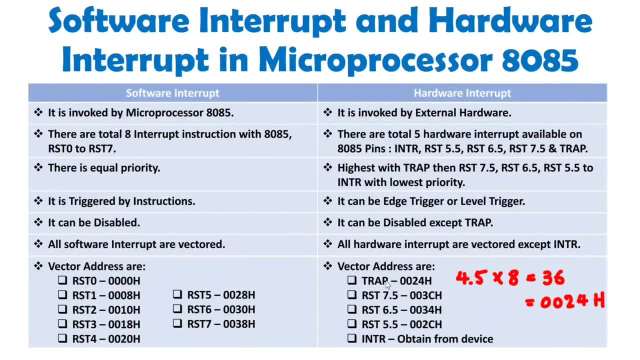 eight, That will be 36, and 36 in terms of hex, that will be 24 hex. Now you see RST: 7.5, 6.5 and 5.5.. That is having these addresses. How to remember this. 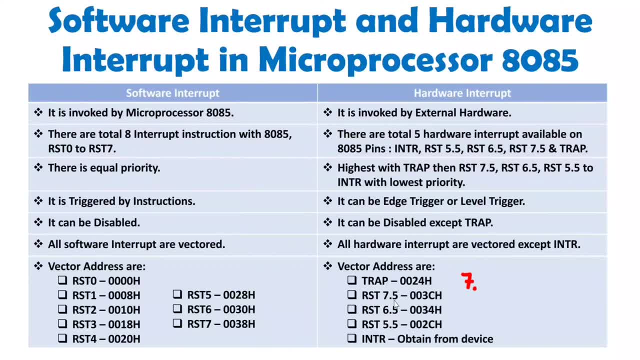 So you don't need to remember direct data: 7.5.. by 8, whatever data comes in terms of hex, it will be 3c. So that is how you can have 6.5 address. that is 3, 4. you just do that. I am just giving it to you in practice: 6.5 multiply by 8 in terms of.